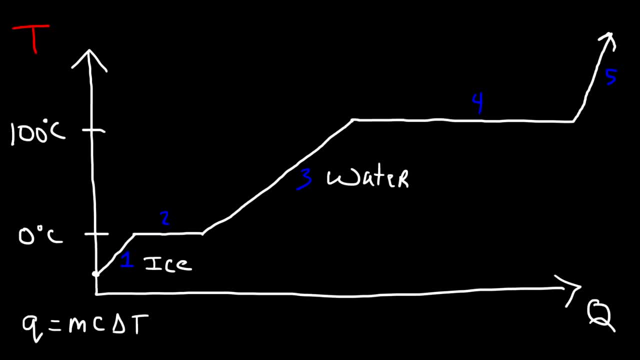 liquid water. now, to calculate the heat energy absorbed as ice goes to liquid water, you can use this equation: Q is equal to the number of moles times the enthalpy of fusion, which is usually in kilojoules per mole. now the enthalpy of. 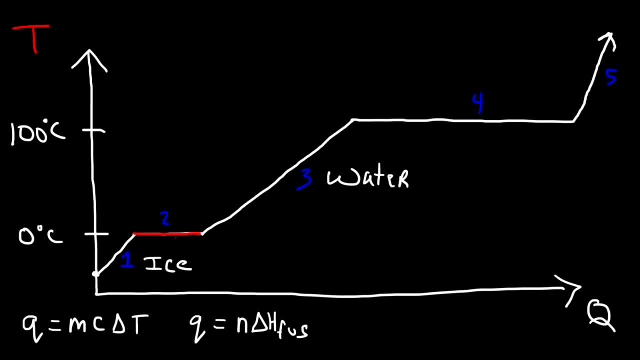 fusion is proportional to the length of this segment. number four represents the enthalpy of vaporization. the enthalpy of fusion for ice is about six kilojoules per mole and the enthalpy of vaporization for water 40.7 kilojoules per mole. so if we divide 40.7 by 6 you'll get like 6.8. so the 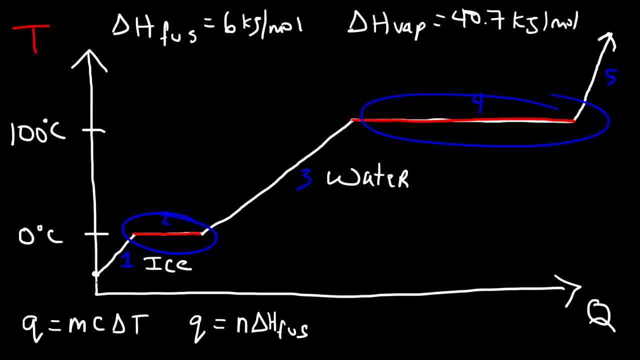 length of this segment should be 6.8 times the length of that segment now granted. my graph is not drawn to scale, but that's the way it should be so during segment 2, the heat energy that's added is converting ice to liquid water, and the temperature is constant during a phase change. now, during segment 2, the 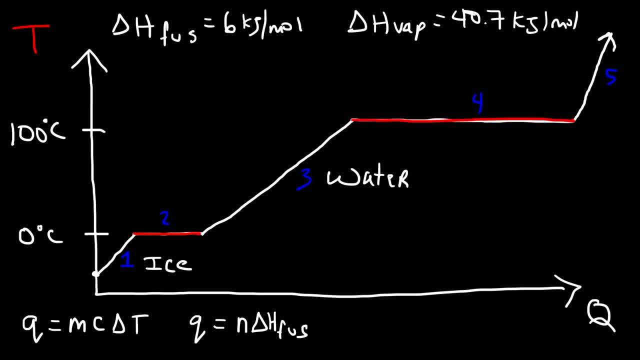 energy that's added doesn't go into the kinetic energy of the molecules because the temperature is constant. kinetic energy and temperature are proportional with regard to gases and liquids, and solids as well. so what is the energy going to be during segment 2? in segment 2, when a temperature is constant, and if you're adding energy to, 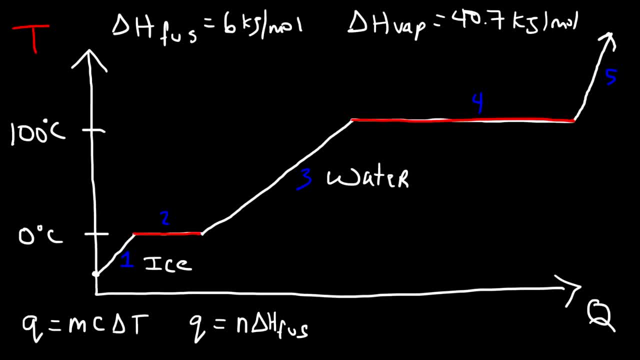 the system. you're not increasing the kinetic energy, rather you're increasing the potential energy. so in segments 1, 3, and 5 the kinetic energy is increasing because the temperature is going up, but for segments 2 and 4 the potential energy is increasing. 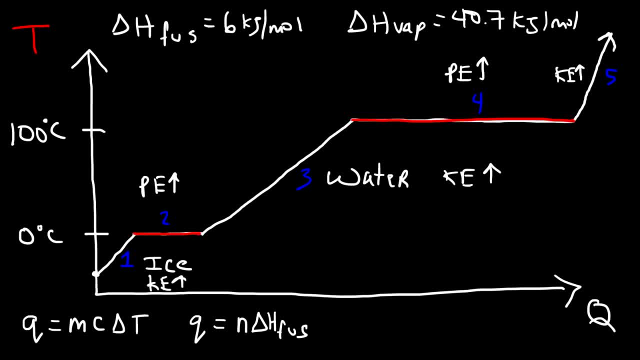 and that is the energy stored in the bonds. so when you heat up ice, you're causing the bonds- the hydrogen bonds- to break, and so you're increasing potential energy. and when you heat up liquid water and turn it into steam, the water molecules are moving further away from each other, and so you're increasing the. 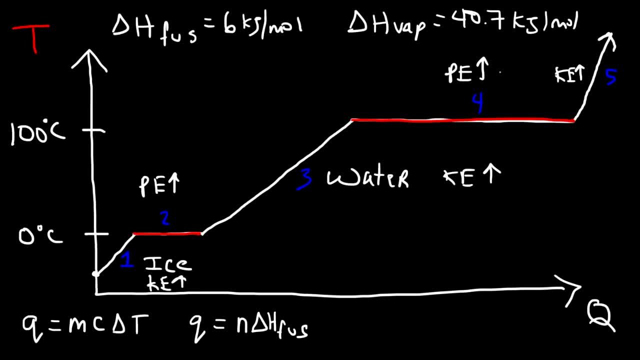 potential energy of the system. when the water molecules come together to form a hydrogen bond, energy is released, and that occurs during condensation. but when you're so, if you add an energy to break the bonds, to break the hydrogen bonds in separate the water molecules, then energy is absorbed to do that, and so 450 is an endothermic process. 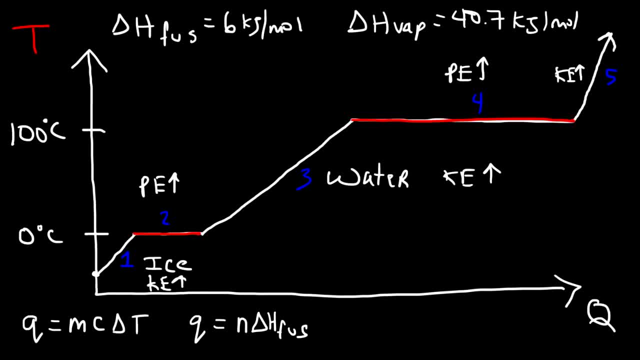 the connotation isn't X. with a process going in this direction, liquid water is vaporizing into steam. So segment five is it's steam, where segment 3 is liquid water. so $��ễzd strength value estimated for 560 ticket value up toa also became wärkat. 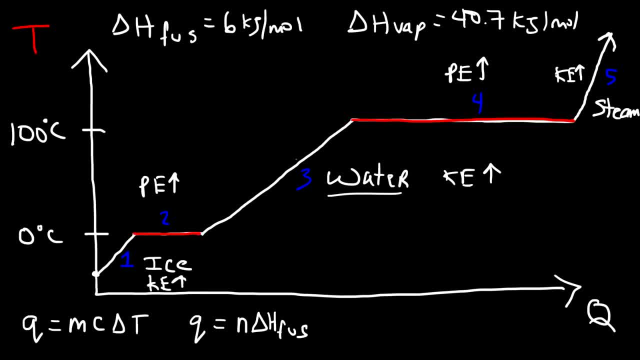 8000 et wo 4 200. For segments 2 and 4, where a phase change is occurring, to calculate the energy for that segment, you need to use this equation. And for segments 1,, 3, and 5, you need to use this equation when there's a temperature change. 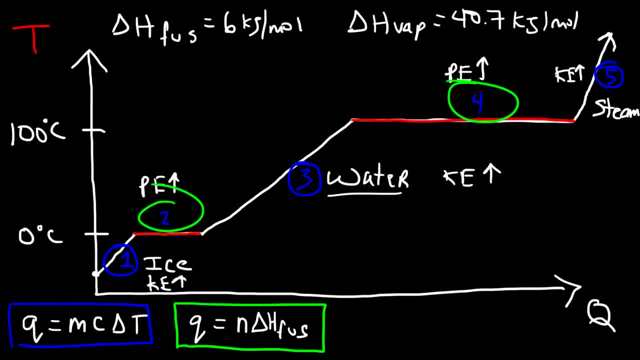 So if you want to find out how much heat energy is required to melt ice all the way to steam, then you need to add up the five Q values for each segment: The energy for segment 1,, 2,, 3,, 4, and 5.. 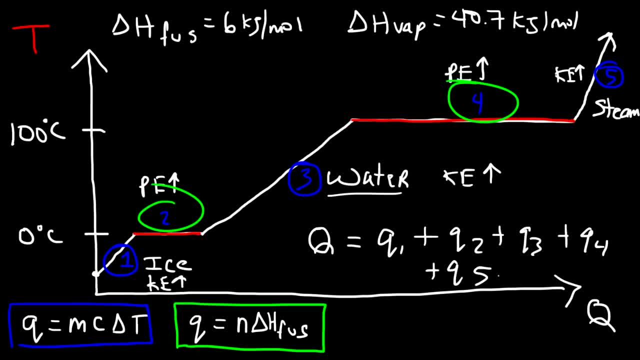 Now the last thing we need to talk about is the slope: The slope of segments 5, 3, and 1.. Notice that the slope of segment 3 is not as high as segment 5 or 1.. And that's due to the specific heat capacity of water. 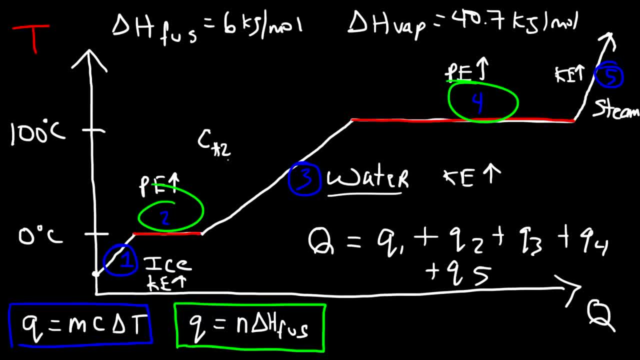 The specific heat capacity of water is the energy for segment 3.. The specific heat capacity of liquid water- I'm just going to put L for liquid- is about 4.18 joules per gram per Celsius. The specific heat capacity for steam is about 2 joules per gram per Celsius. 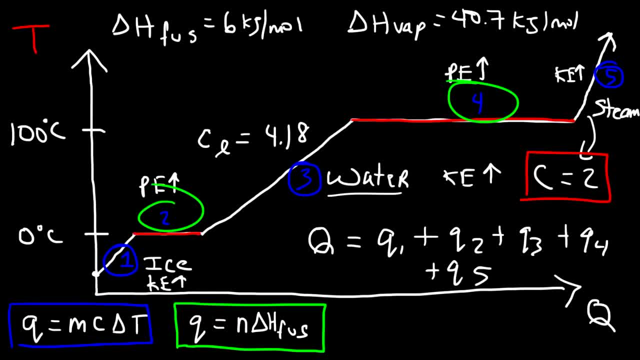 So notice that a substance with a low specific heat capacity, or a phase with a low specific heat capacity, has a very steep slope, And a substance with a relatively a relatively high specific heat capacity has a slope that's not as much or that's lower. 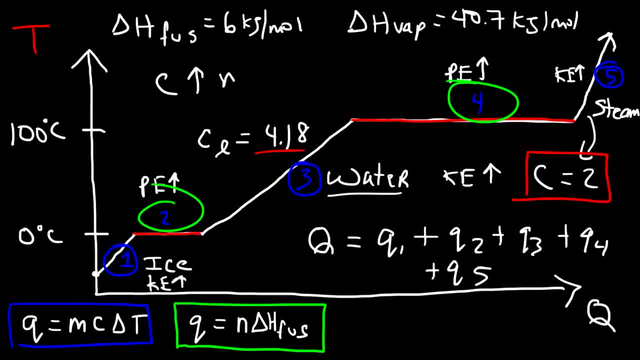 So as the specific heat capacity increases, the slope of the line decreases. They're inversely related And it makes sense. The specific heat capacity of water is so high because water can absorb a lot of heat energy without increasing its temperature much. It takes 4.18 joules of heat energy to heat up 1 gram of water by 1.7 degrees. 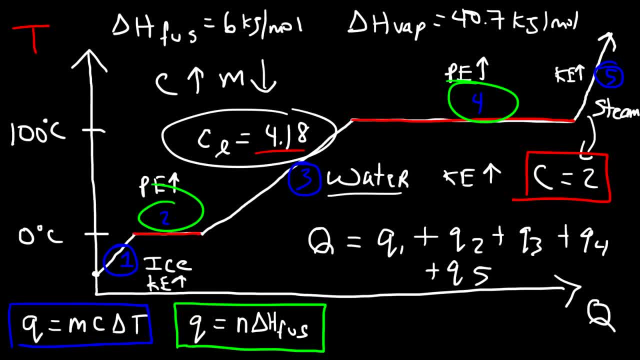 In the case of steam, it only takes 2 joules of heat energy to heat 1 gram of steam by 1 degree Celsius. So therefore, let's say, if you add about 8 joules of heat energy to 1 gram of liquid, 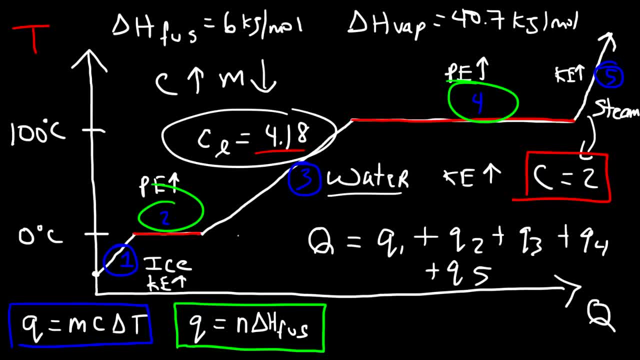 water, the temperature would go up by approximately 2 degrees Celsius- A little bit less, but I'm just going to round it Now. if you add 8 joules of heat energy to steam, the temperature would go up by approximately 2 degrees Celsius. 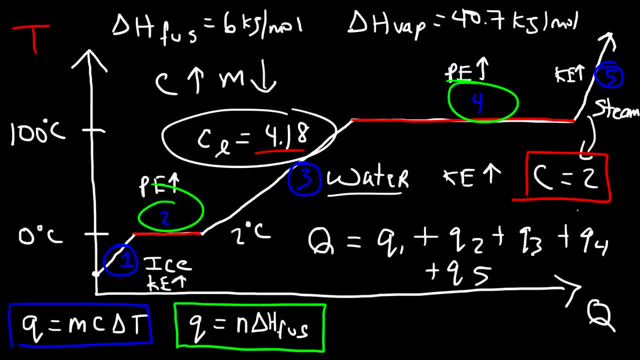 Let's say 1 gram of steam, the temperature will change by 4 degrees Celsius. It's 8 divided by the heat capacity, 2, which is 4.. So when adding the same amount of heat, the temperature of water changes less than the. 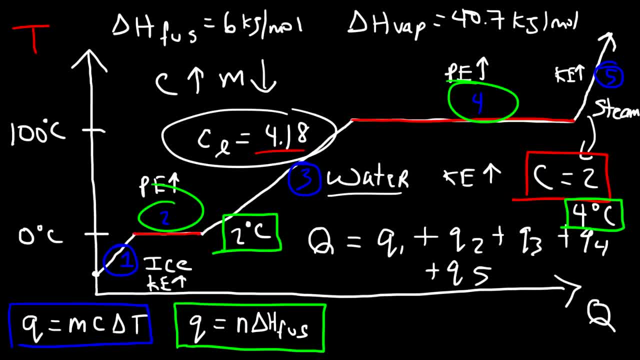 temperature of steam And that's why the slope is less, Because it takes a lot more energy to heat up water than it does steam. So make sure you understand that substances with a very high specific heat capacity will have a low slope and represent slope. 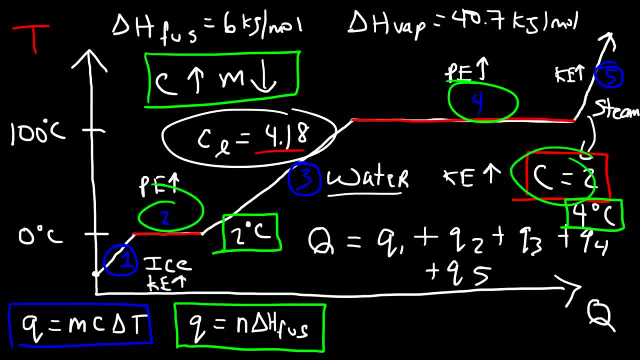 And substances with a low specific heat capacity will rise up quickly. The temperature will change a lot faster for substances with a low specific heat capacity, Whereas a substance with a high heat capacity, the temperature doesn't change as rapidly. Now let's talk about the cooling curve of water. 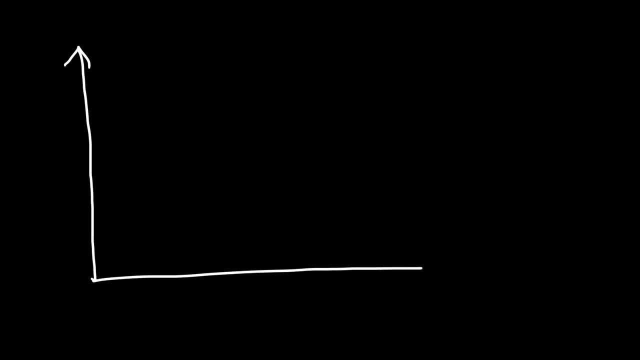 So the heating curve is an endothermic process, But the cooling curve is an exothermic process. So when dealing with the heating curve, you're starting from a low temperature and gradually you're going to increase towards a high temperature. With the cooling curve you're starting from a high temperature and you need to decrease. 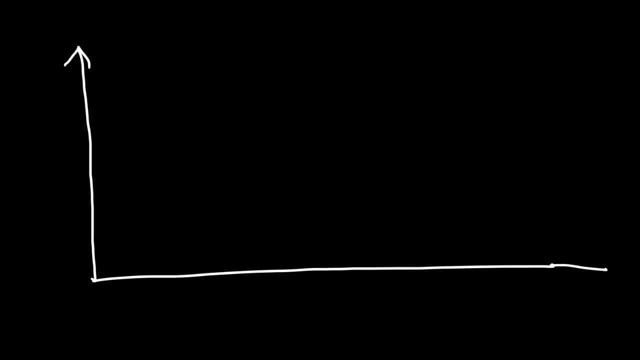 towards a low temperature. So once again we're going to have temperature on the y-axis and the amount of heat energy added on the x-axis. So let's say this is 100 degrees Celsius And this is going to be 0 degrees Celsius. 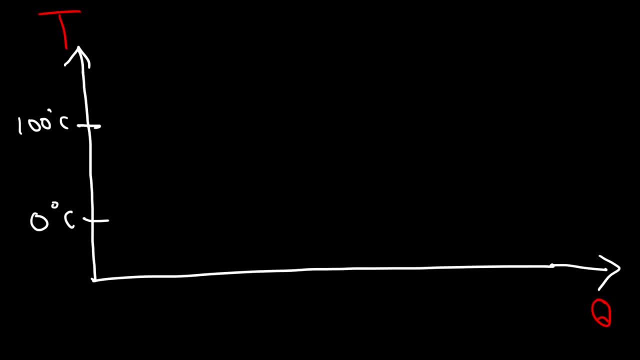 So we're going to start with steam at this point And the slope should be very steep, And then it's going to take a lot of energy, or a lot of energy will be released as steam condenses into liquid water. So I'm going to make that line very long. 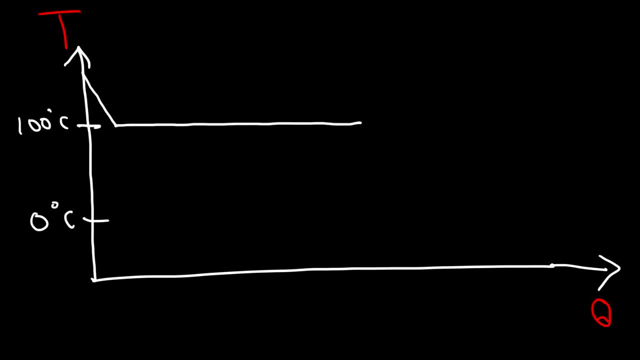 Now, as the temperature of water decreases, we know water has a very high specific heat capacity, So the slope shouldn't be as steep as what we have here. So this is going to be 0 degrees Celsius, So we're going to start with steam at this point. 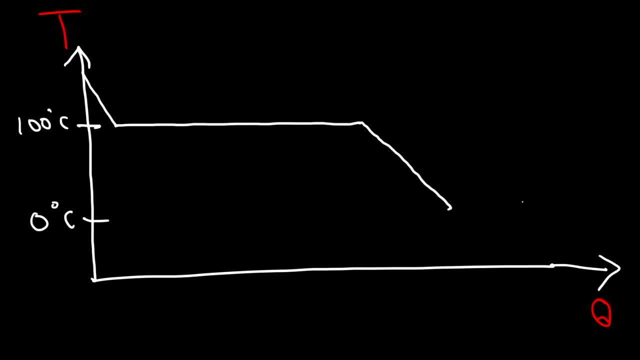 This is going to decrease gradually, And then the enthalpy of vaporization- I mean for fusion- is much less than the enthalpy of vaporization. So this line has to be 6.8 times longer than this line. So I'm going to make this line very small or very short. 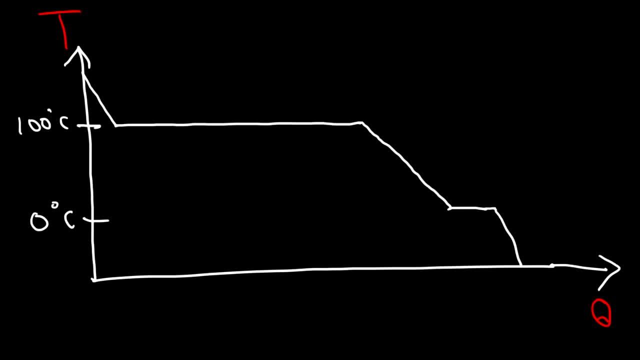 And then this is going to decrease rapidly. The specific heat capacity of steam is very close to the specific heat capacity of liquid water, So these two lines should be very steep. They're both around 2 joules per second, 2 joules per gram per Celsius. 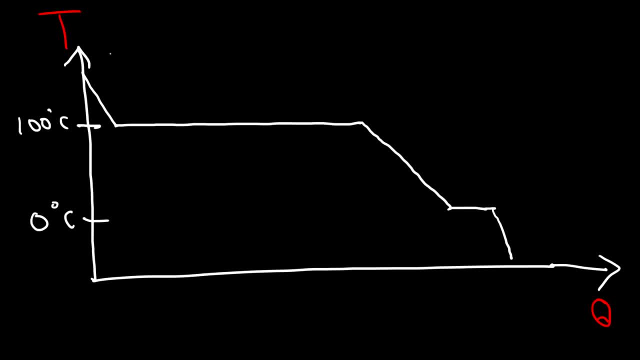 But this line shouldn't be as steep, So the slope of these two lines should be twice as much as the slope of that line if you want to draw it accurately. So this is segment 1,, 2,, 3,, 4, 5.. 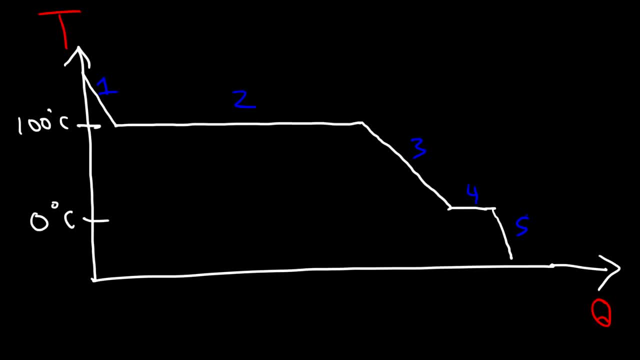 So this entire cooling curve is an exothermic process. Energy is being released In segment 1, steam is losing kinetic energy. So this entire cooling curve is an exothermic process. Energy is being released. Steam is losing kinetic energy. 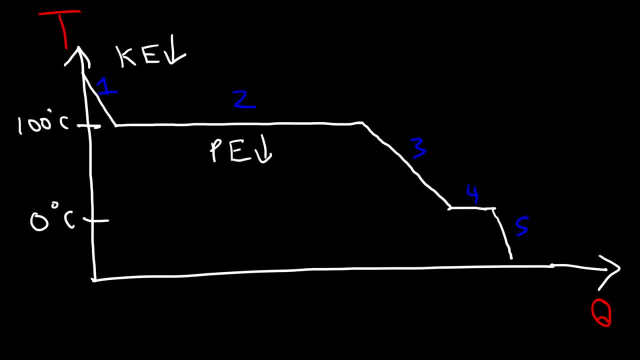 In segment 2, it's losing potential energy. As the steam molecules or the water molecules in steam, they're approaching each other, And as they approach each other, they begin to form a hydrogen bond. Whenever a bond is formed, energy is released. 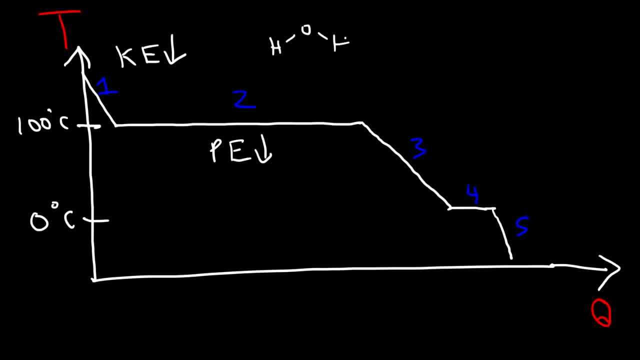 So in segment 2, let's say this is a water molecule In the gas phase. it's very far apart from another water molecule. But as these two molecules approach each other they begin to form a hydrogen bond, And when that bond is formed, energy is released. 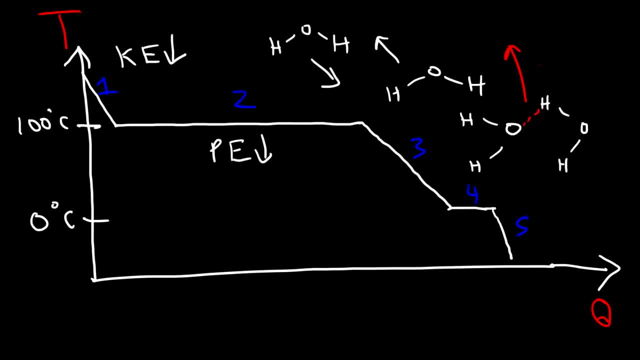 To form a bond, you've got to put in energy, But to form a bond, that's an exothermic process. it releases energy. So that's what's happening in segment 2. The water molecules are approaching each other, forming that hydrogen bond and the potential. 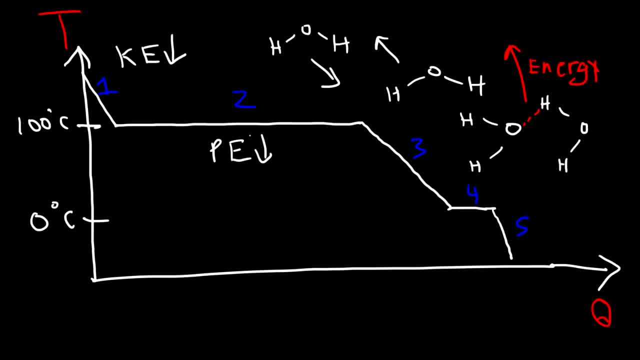 as thermal energy. So the potential energy of the system decreases and it's released as heat energy into the surroundings. Now, in step 3, the system being the water- loses kinetic energy. and in step 4, it loses potential energy as the liquid water molecules freeze into ice. and in step 5, it loses kinetic 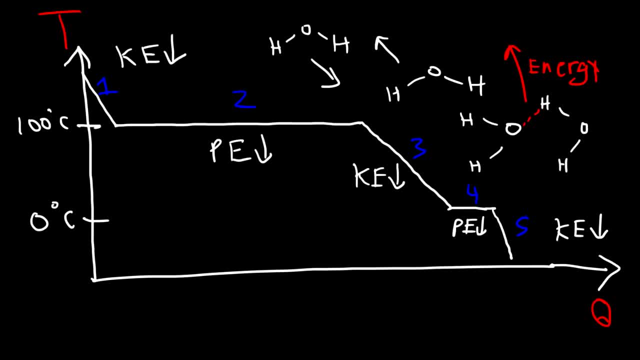 energy. So notice that a temperature change is associated with a change in kinetic energy, So that's in segments 1, 3, and 5. And a phase change is associated with a change in potential energy, So kinetic energy has to do with energy in. 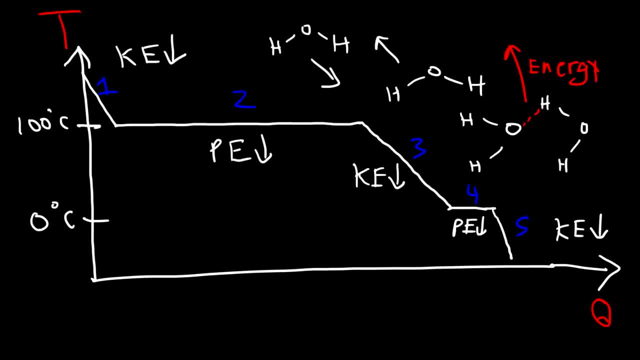 motion. The higher the temperature, the faster the molecules are moving. So for a gas phase, a high temperature means that the gas is moving with a greater velocity, so they have more kinetic energy. In terms of a solid, a higher temperature means that the solid is vibrating at a greater rate. But 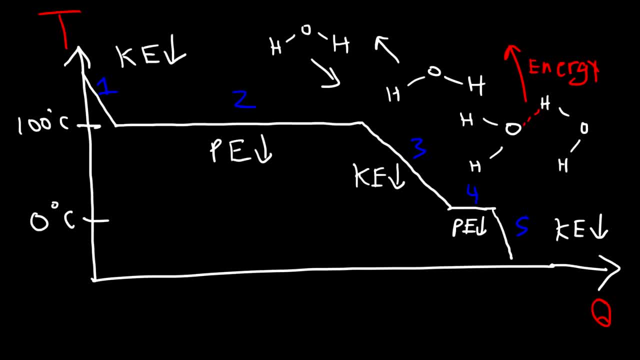 you're still dealing with motion, so you're dealing with kinetic energy, And so that's about it for this video. I believe we've covered everything else. You know that Q2 and Q4 can be calculated using this equation. It's the moles times. 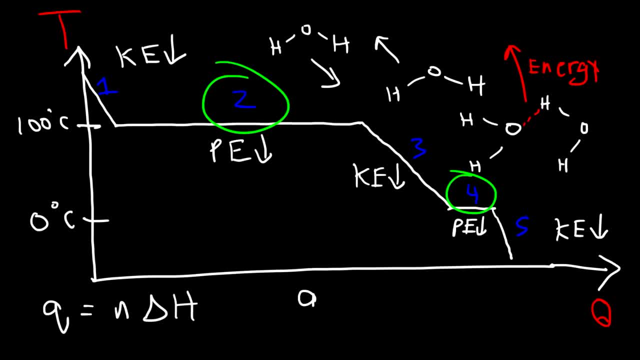 the enthalpy and Q1,, Q3, and Q5. they can be calculated using this equation: MC, Delta T. So the cooling curve is simply the reverse of the heating curve. So that's it for this video. Thanks for watching and have a good day. you.